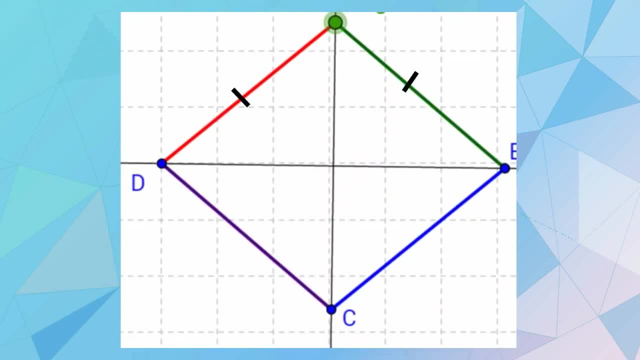 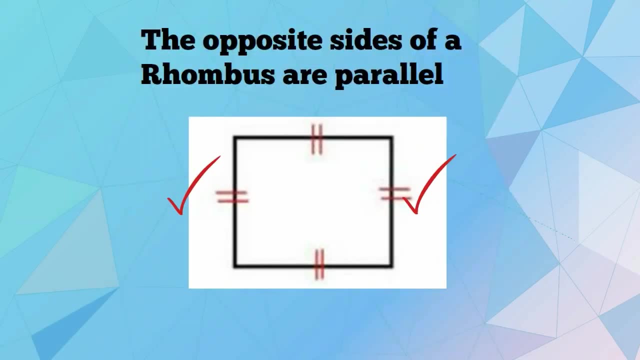 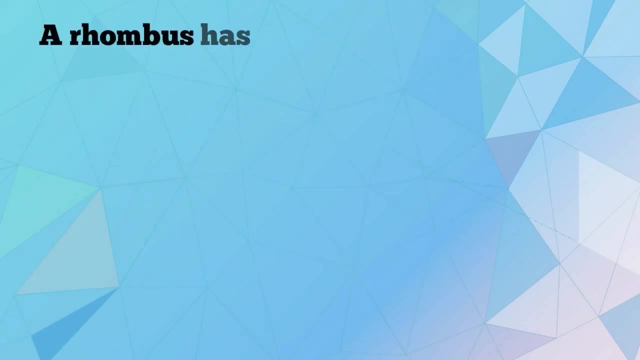 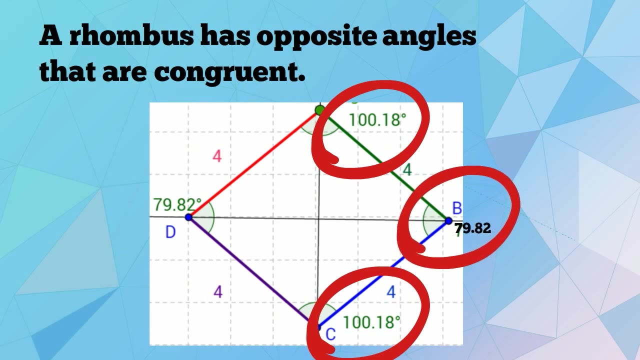 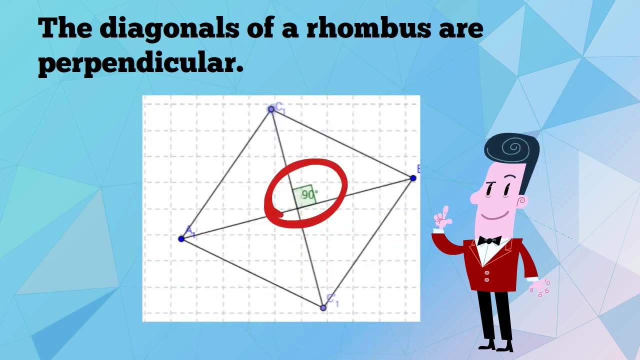 or equal. The opposite sides of a rhombus are parallel. A rhombus has opposite angles that are congruent. The opposite sides of a rhombus are parallel. A rhombus has opposite angles that are equal. The diagonals of a rhombus are perpendicular. This means the Getting. 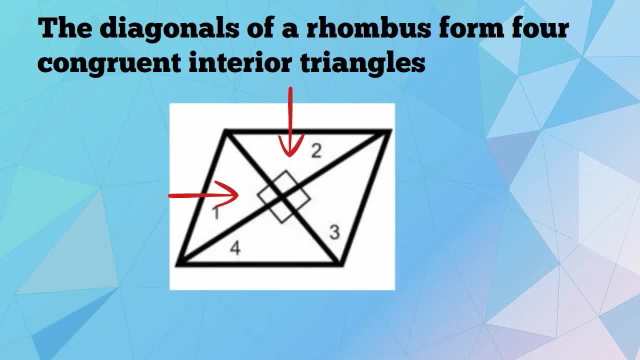 Right Angle downside is not perpendicular. The diagonals of a rhombus form four congruent interior triangles. The diagonals of 2 Por impacting in the 6 basic pieces are rather unique. Starting with the base of the rhombus, The diagonals 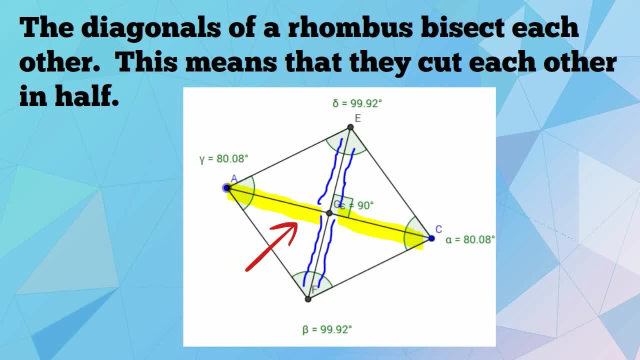 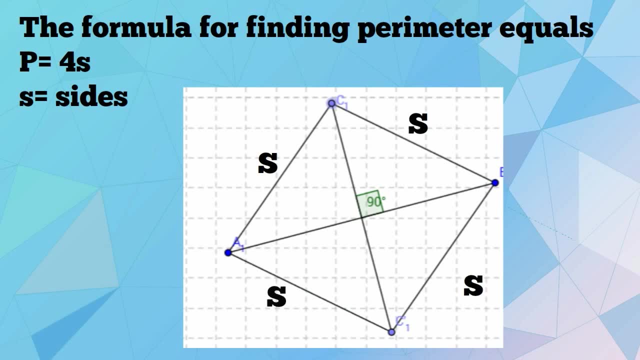 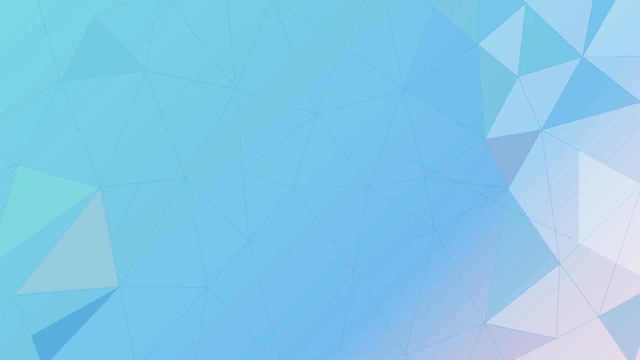 of a rhombus bisect each other. This means they cut each other in half. Formula for Finding the Perimeter of a Rhombus gre sand p, 4 s, 3 sides. The formula for area equals 1 half diameter 1 times diameter 2.. 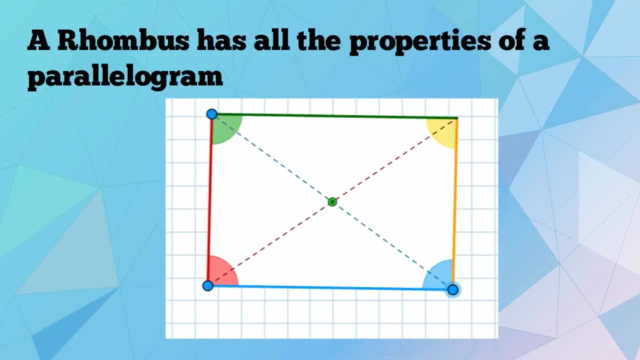 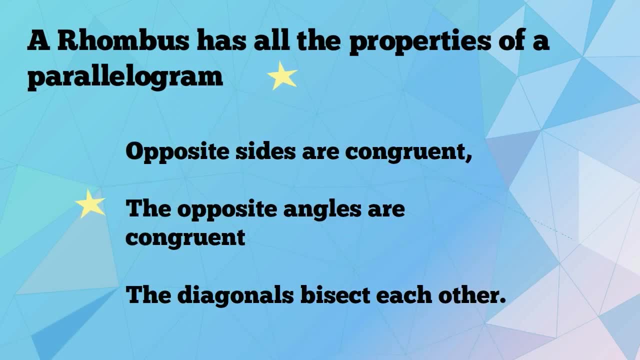 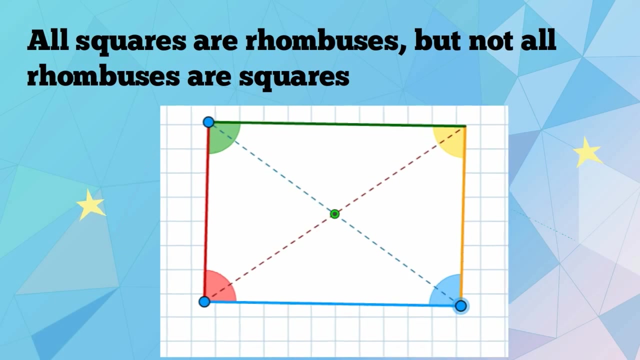 A rhombus has all the properties of a parallelogram. These include: Opposite sides are congruent. Opposite angles are congruent. Diagonals bisect each other. All squares can be considered a rhombus, but not all rhombuses are squares. 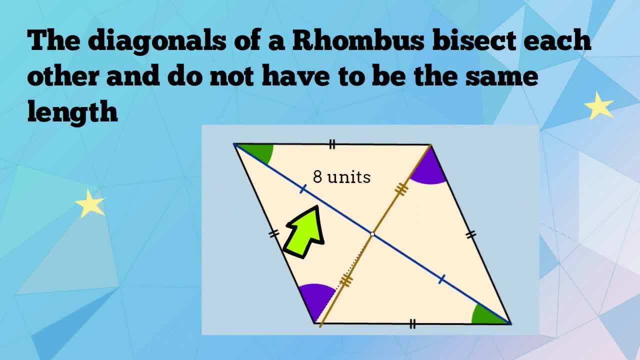 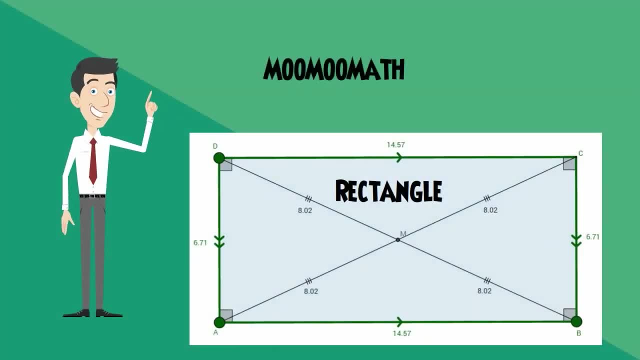 The diagonals of a rhombus bisect each other, but they do not have to be the same length. Hello, welcome to MooMooMath. In this video I'd like to talk about the properties of a rectangle. A rectangle is part of the quadrilateral family. 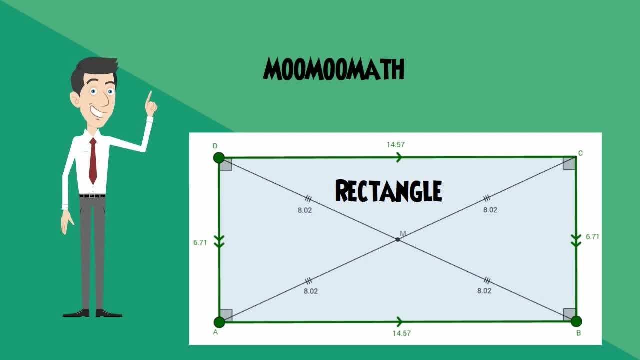 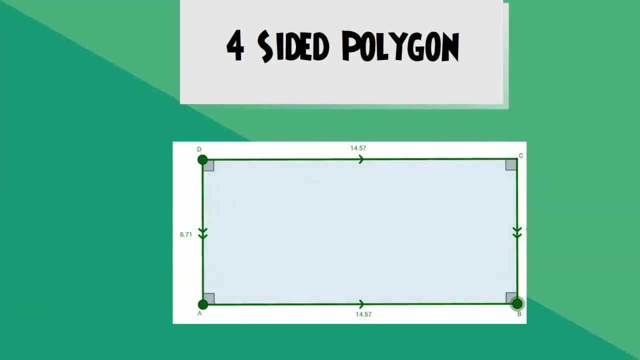 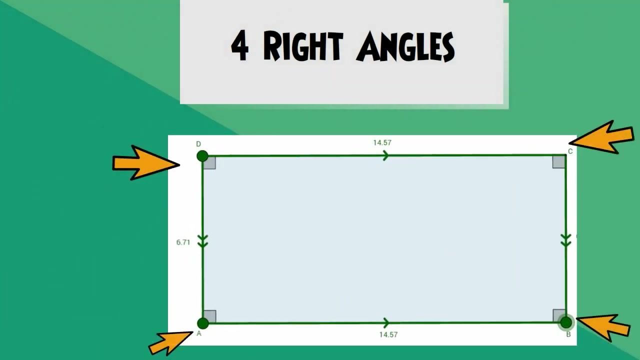 This means it is a plane shape with four sides. In addition, it has several other properties. A rectangle is a four sided polygon, with opposite sides being parallel. In addition, a rectangle has four right angles and the sum of these interior angles add to 360 degrees. 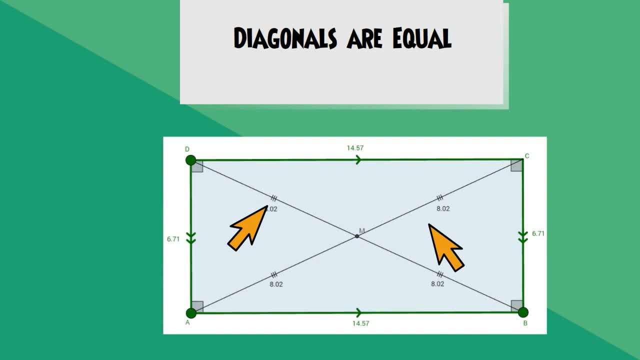 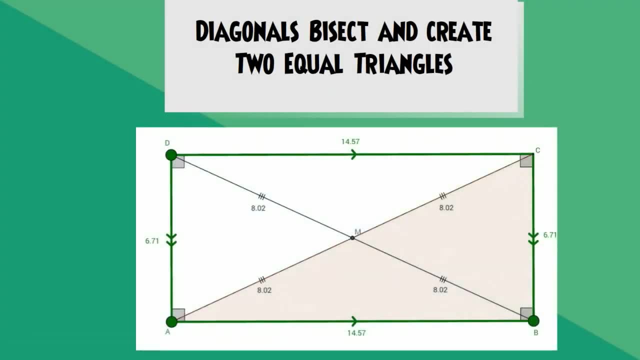 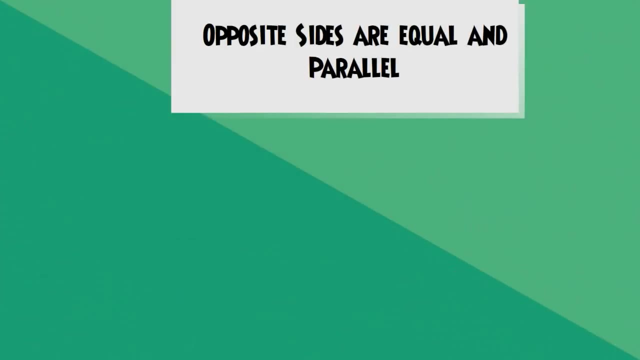 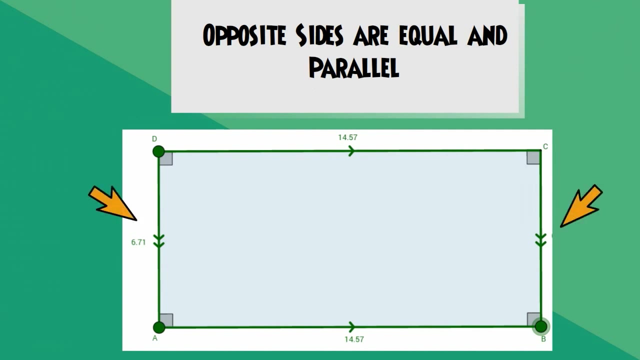 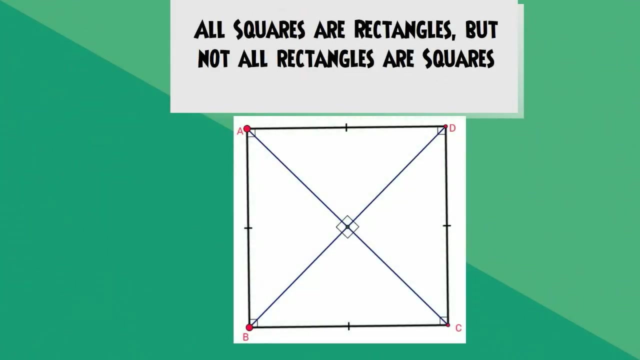 Lets talk about the diagonals of a rectangle. The diagonals of a rectangle are of equal length. The diagonals also bisect and create two pairs of equal triangles. Opposite sides of a rectangle are equal. Both sides are parallel. All squares are rectangles. 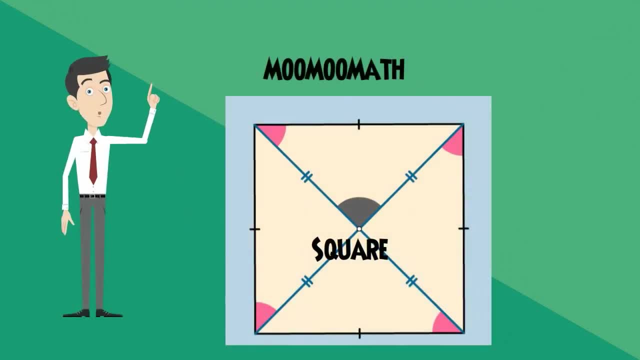 But not all rectangles are squares. Hello, welcome to MooMooMath. In this video, I would like to talk about the properties of a square. A square is a plane shape. It is a quadrilateral that is two dimensional, So it has length and width, but not height. 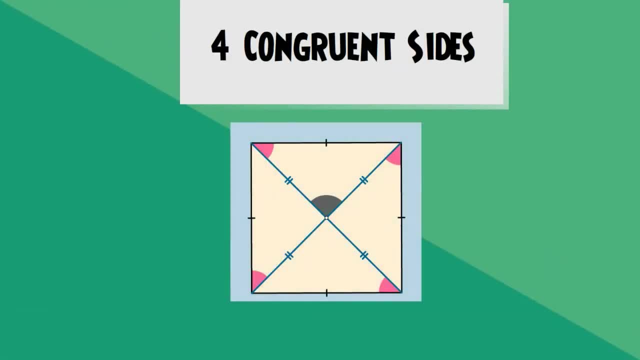 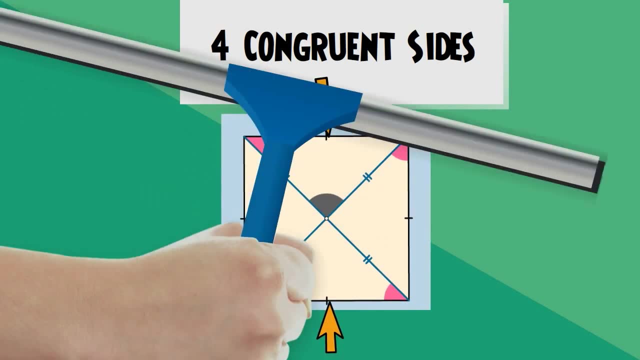 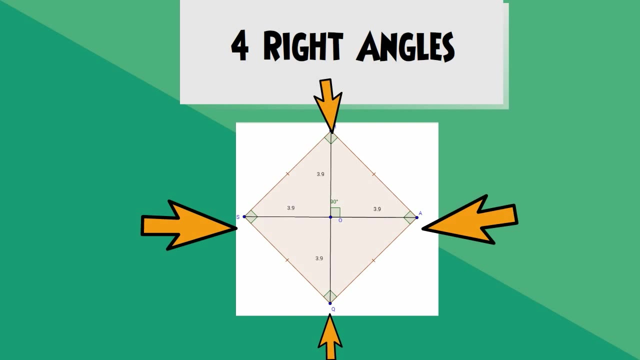 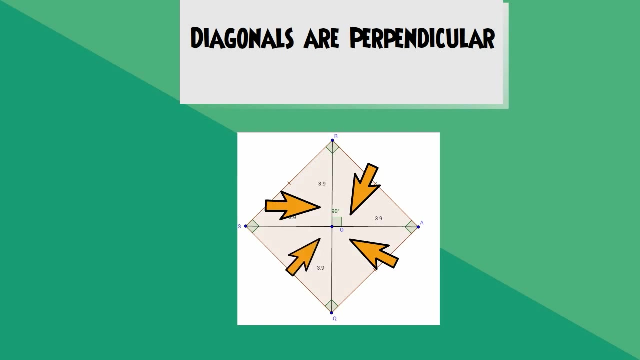 Excuse me, It is a quadrilateral, It is a square. A square has four congruent sides, four equal sides. Along with these four sides, you have four right angles. The diagonals of a square are perpendicular and create four right angles. 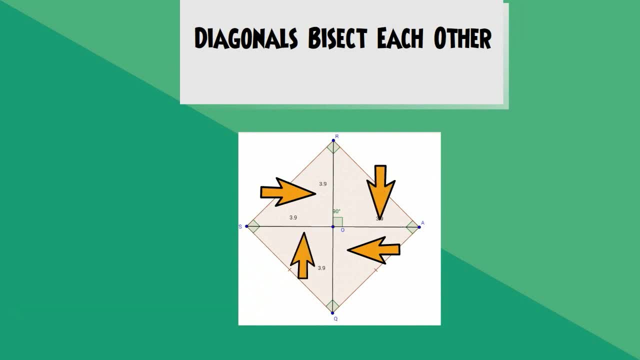 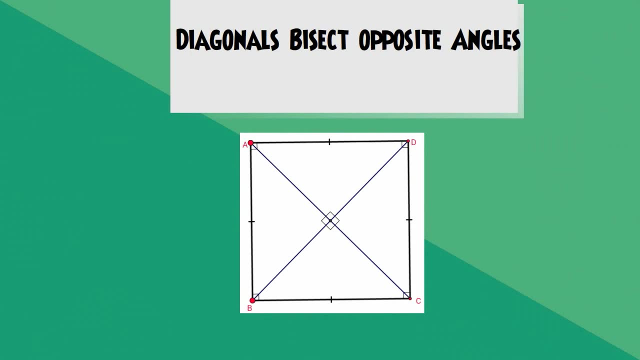 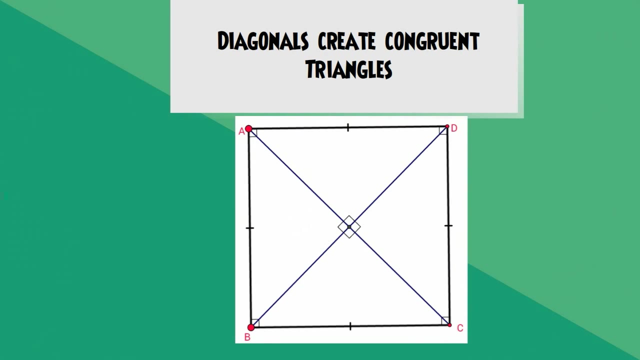 The diagonals also bisect each other. Diagonals also bisect opposite angles and create equal 45 degree angles. As a result of the diagonals bisecting opposite angles, they create triangles that are congruent: Triangle a, b and c.